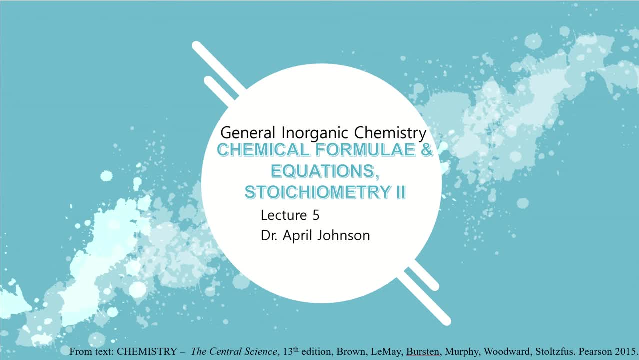 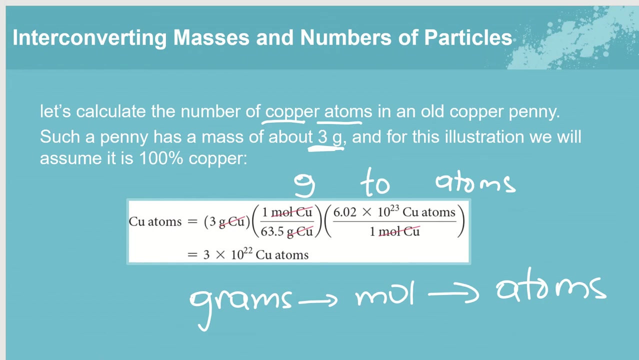 Hi guys, welcome to another lecture in the series General Inorganic Chemistry, and today we'll be continuing our conversation about chemical formulae and equations, as well as stoichiometry. So in continuing these types of calculation, we're going to proceed with into converting masses and numbers of particles. So let's start off with a question. It says: 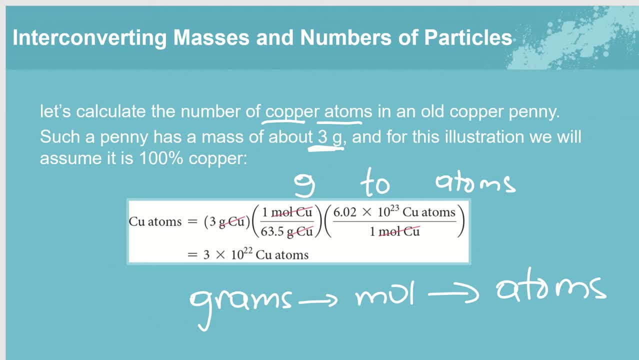 let's calculate the number of copper atoms in an old copper penny. Such a penny has a mass of about three grams and for this illustration we will assume it is 100% copper. So here we have our equation. So, if you recall from our previous calculations, we have our given unit, which is in. 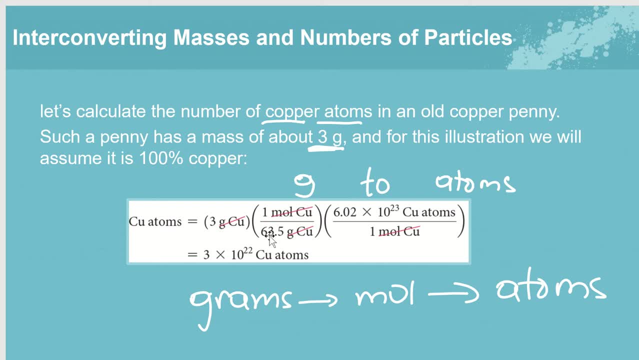 grams, and we have our desired unit in the first set of conversion factor. here We're converting grams to moles, and then for the second conversion factor, we're converting moles to atoms, right? So essentially, we're going from grams to moles, to atoms, right, and so that is. 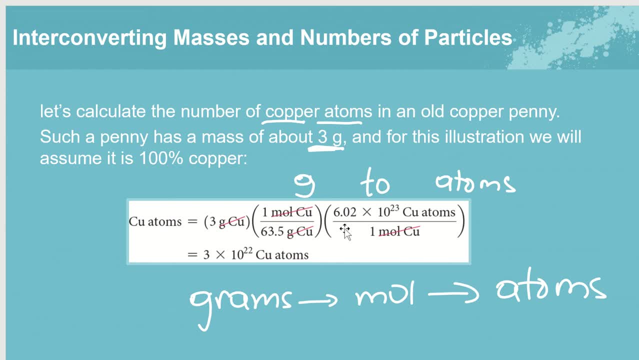 why we have two different conversion factors. So, essentially, the unit that we're trying to get rid of is normally in the denominator and the desired unit is usually in the numerator right. So this is the first conversion, and then for the second conversion, to atoms, the same is true. So the 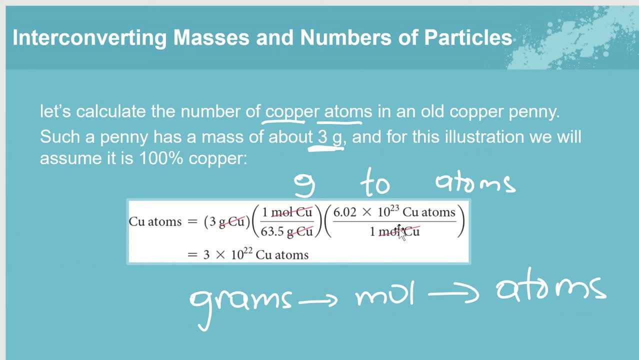 unit that we're trying to get rid of is in the denominator and the desired unit, which is atoms, is in the numerator right. So essentially, we just carry out this calculation from grams to moles, to atoms, and then we're going to convert the number of copper atoms in the denominator. So this is. 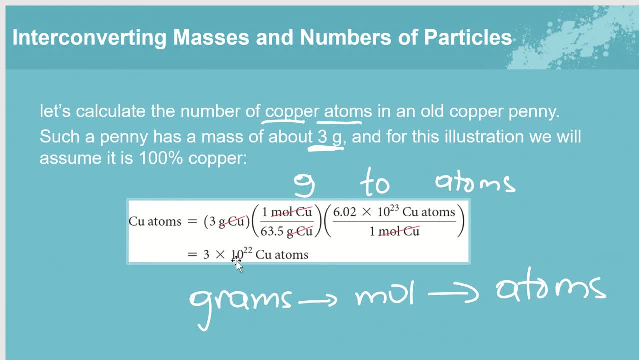 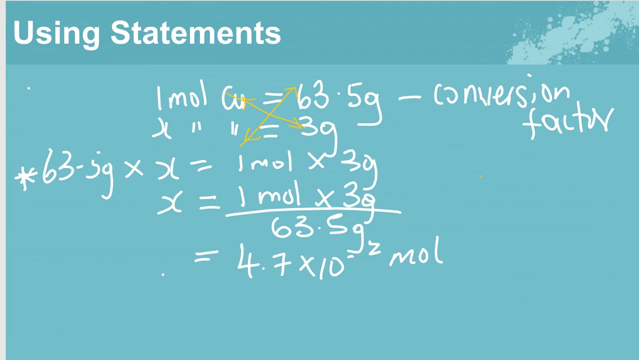 the first conversion and then, once we do that, and we should get three times ten to twenty two copper atoms, right? So go ahead, plug the values in your calculator and see if you get the same answer. So I like to do the same calculation using statements, right? because that way we show that we understand fully. 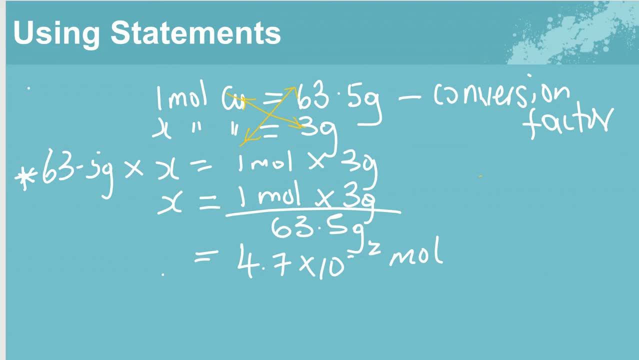 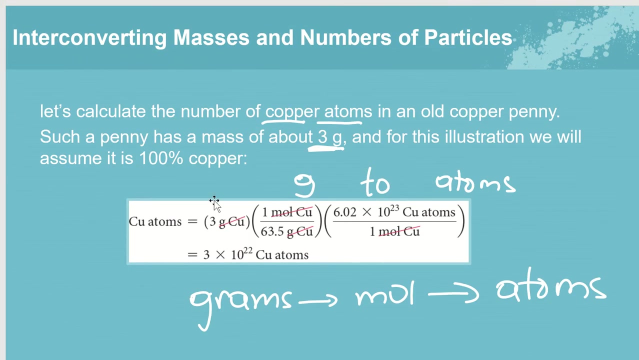 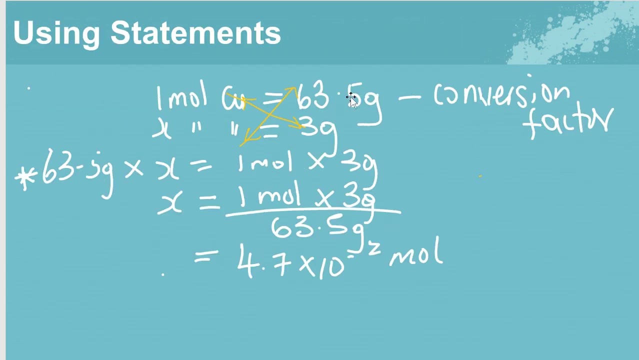 what is happening. We're not just plugging in values into an equation, right? So let's do the same calculation using statements. So we have to have, in a similar fashion, our conversion factor. So remember, here we have our two conversion factors. Yes, we're going to use them as well. So our first, 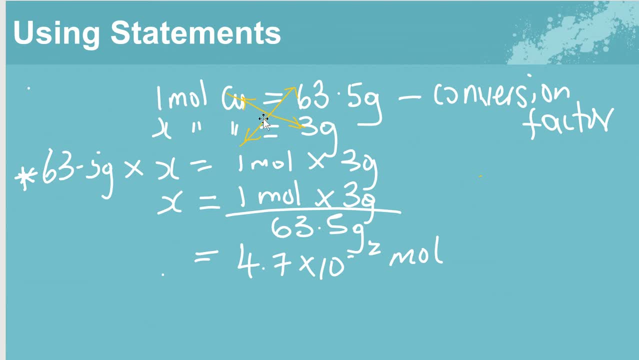 statement is that one mole of copper is equal to sixty three point five grams, and that is our conversion factor. So remember, guys, your conversion factor has both units right. It has your given units and your desired units. So remember, for the first calculation we're going from grams to moles, and so our conversion factor must have a true. 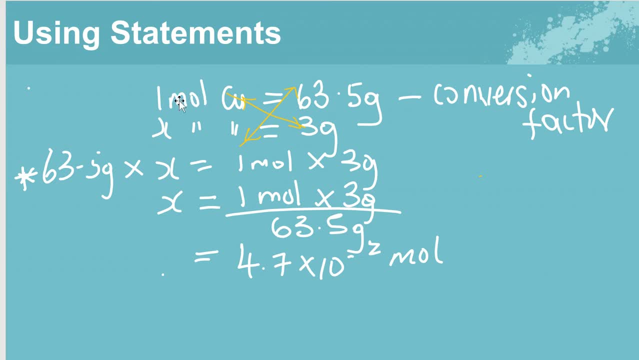 statement Which has both mole and gram right. And so here we cross multiply right. And so once we cross multiply, as we see here, and then we make x the subject of the formula right, by dividing both sides by sixty three point five, And you know, carrying out this calculation, we get moles. 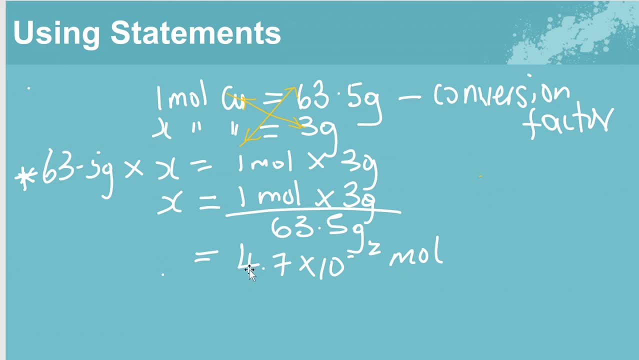 Right. So here we have the value of the value of the moles, which is four point seven times ten to the minus two moles. So what we're seeing here is that one mole of copper is equal to this amount of grams. So if we have three grams of copper, then we clearly would have less than one, significantly less than one mole. 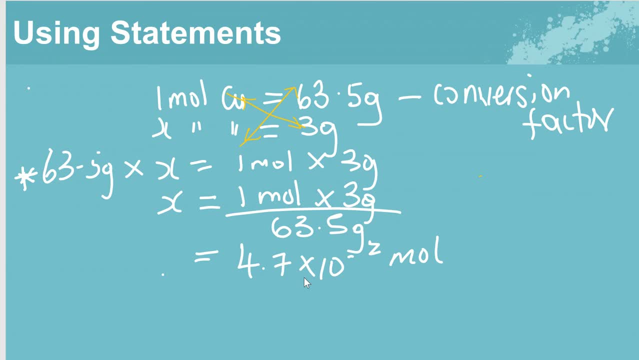 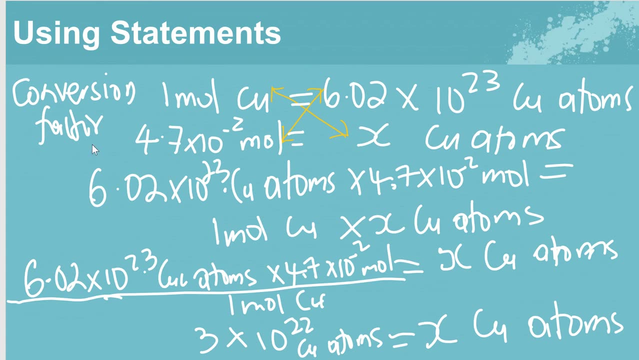 And that's what we're seeing here, seen here in the calculation. all right, so for the second set of calculations, we're going from. what are we going from here? we're going from moles that we just calculated to atoms. right, I know this slide doesn't look the best, but it has. 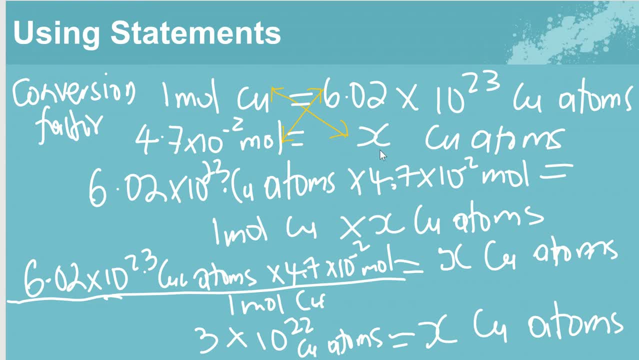 what we need right. and so here X is our unknown, because we are trying to get from moles to atoms. so we have a different conversion factor here. our conversion factor here has moles and atoms, and from our chemistry we know that one mole of copper is equal to six point zero, two times 10 to 23, which is: 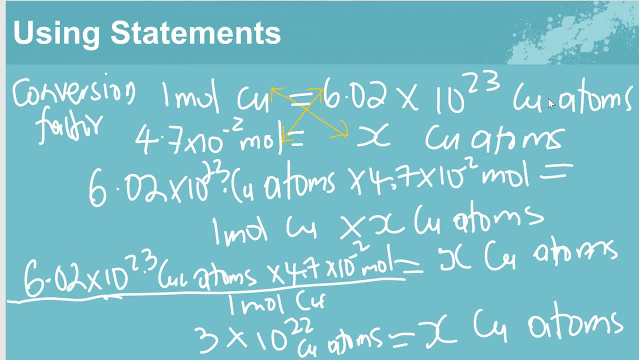 Avogadro's number, copper atoms. so the one mole of copper is equal to the 6,3 point five that we saw earlier, grams, but it's also equal to Avogadro's number of atoms, right, so note: or units, this is atoms, and so in a 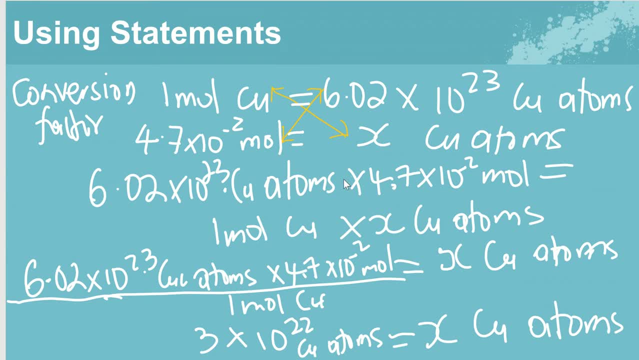 similar fashion, we do our cross multiplication and we make X the subject of the formula as we see here, do our multiplications and division and we end up with 3 times 10 to 22 copper atoms. so I hope that you know. you actually pull out your calculator and do it this way as well. so let's check to see if we have. 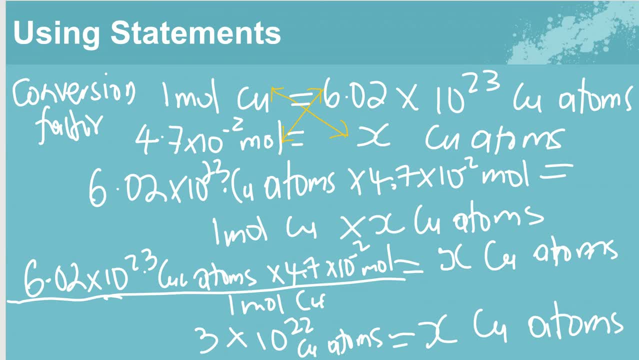 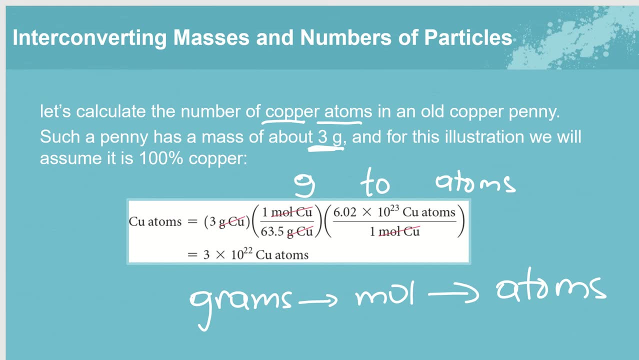 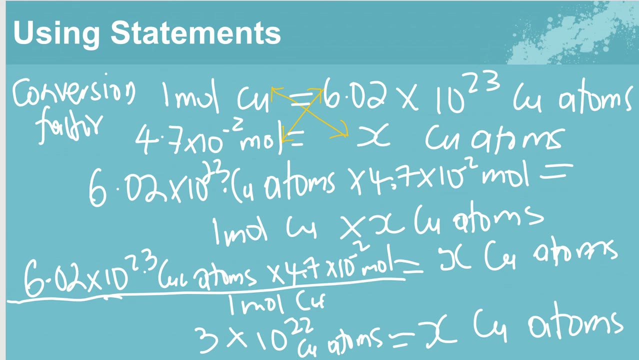 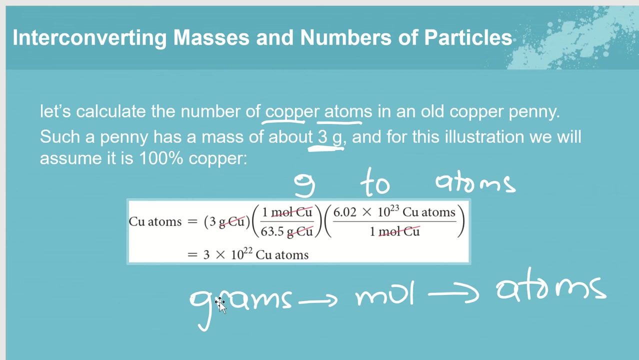 the same answer that we got before. yes, indeed, we have the same answer that we got before, right? so I'm encouraging you guys to use statements, because that will help you to understand what you're calculating and not just plugging in values and not know what you're doing. so just to repeat, here we're going from: 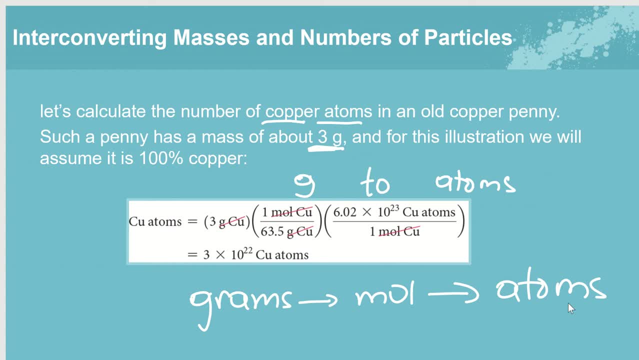 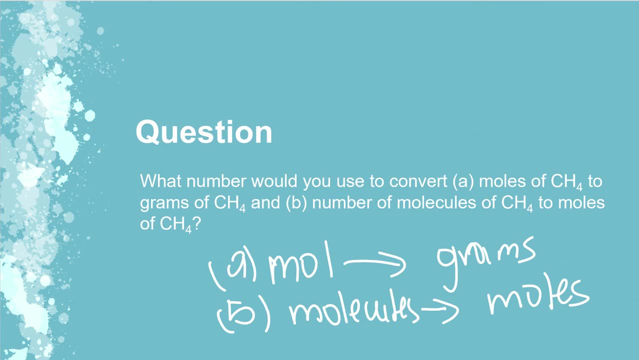 grams to moles and then to atoms. all right, so let's see if we can answer this question. it says: what number would you use to convert moles to grams? right, moles? notice: you're not given any amount of moles or any amount of any grams like. 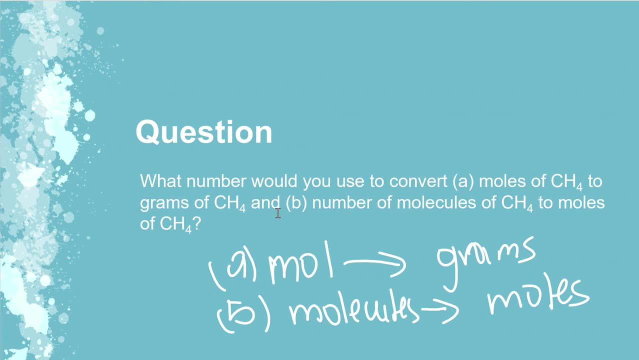 three grams, for example, you're not given. you know, previously we calculated 4.7 times 10 to the minus 2 moles. you're not given any number for those units. so you what the question is asking is: how would you convert moles to grams? essentially like, just generally speaking, that's a and then for Part B it. 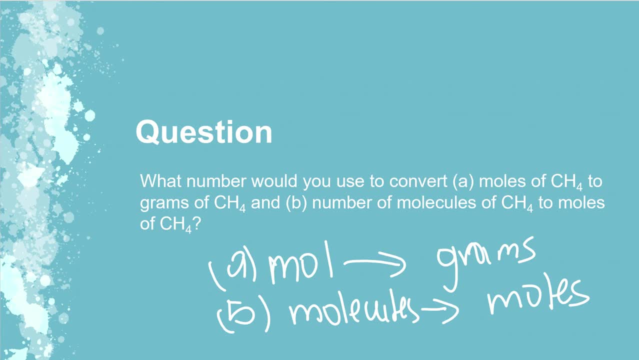 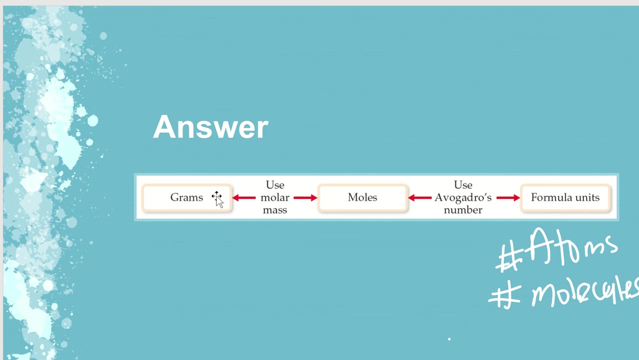 says: how would you convert number of molecules to moles? right? so essentially, for a, we're going from moles to grams, and Part B, we're going from molecules to moles, all right. so if this is what you had, then you are indeed on the right. 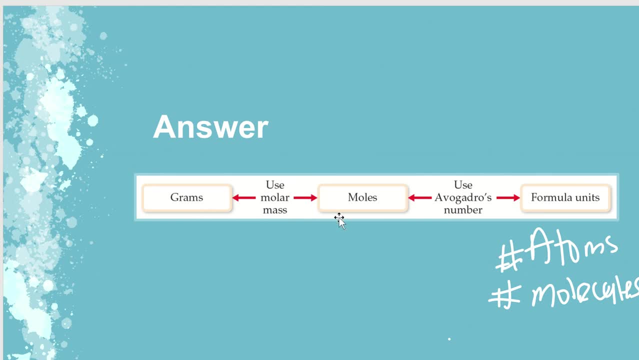 track. so to convert grams to moles or moles to grams, we use the molar mass right, so would have used the molar mass of methane. and to convert moles to formula units. so when we talk about atoms, when we talk about molecules, we use Avogadro's. 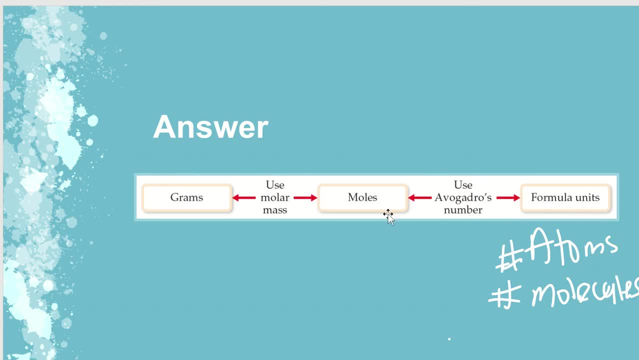 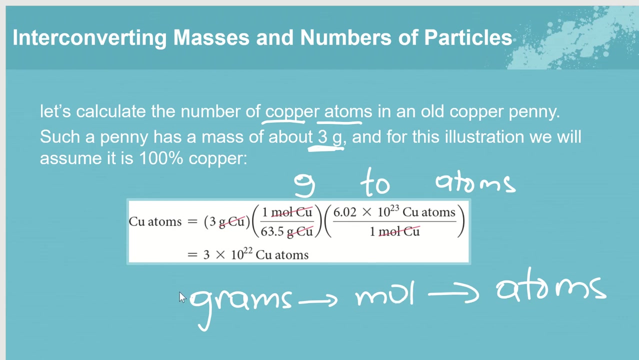 number right. so if we're going from moles to atoms or molecules, for example, we use Avogadro's number. so here in this previous question we were going from moles to atoms. notice, we went from grams to moles, so we use the molar mass and we 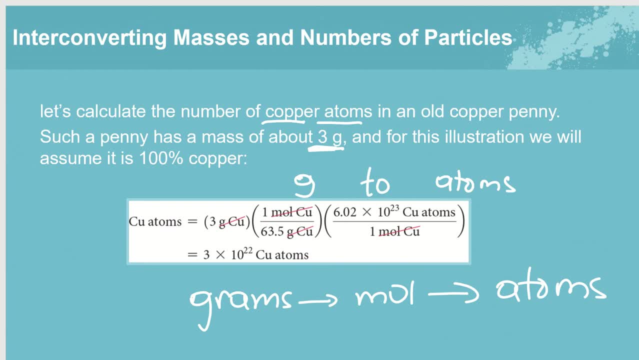 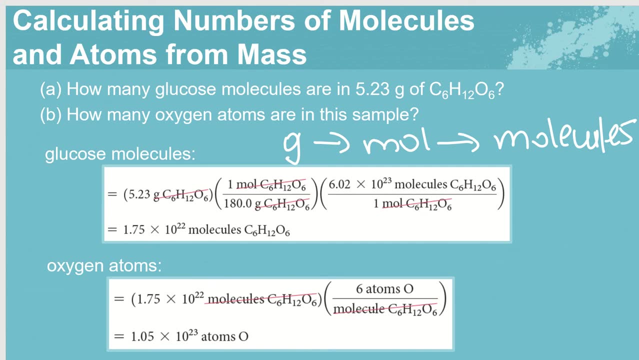 use the Avogadro's number, as seen here. all right. so at this point now we want to talk about calculating numbers of molecules and atoms from mass right? so, as usual, we have a question to help us, to answer or to learn how to do this. So for part A, it says how many glucose molecules are in 5.23 grams of C6H12O6. 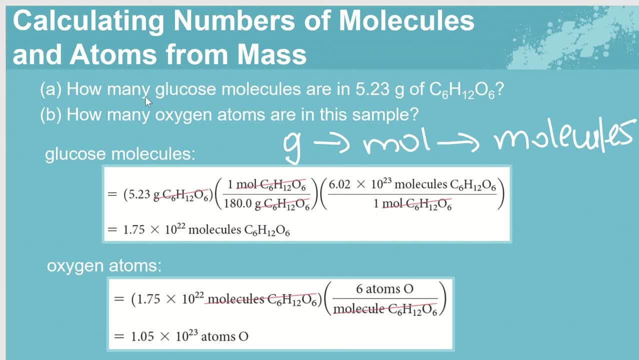 So further on, you will see that I use GLU to signify or to represent glucose, And glucose is the same as C6H12O6, right, So it's the same thing. So how many glucose molecules are in 5.23 grams? 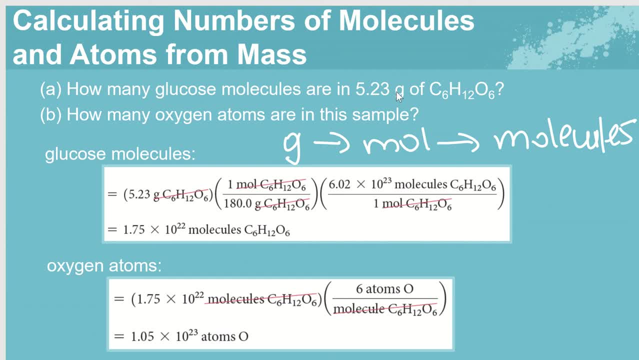 So when you see a question like this, you want to be aware of what you're going from and where you're going, right. So in this case, we're given grams, right, And we're asked- We're asked to calculate molecules. 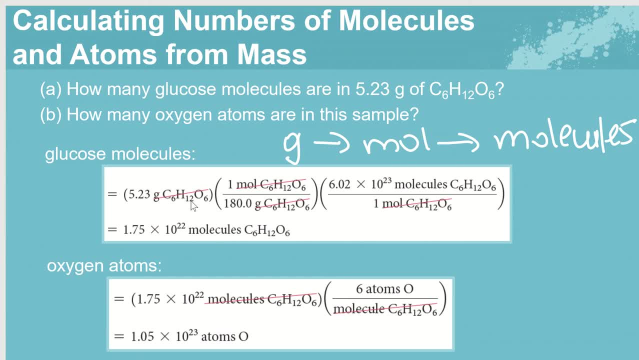 So, in a similar fashion as we saw before, we're going from grams to moles and then to molecules in this case, Because previously we looked at atoms, right Going to atoms, But here we're going to molecules. okay, 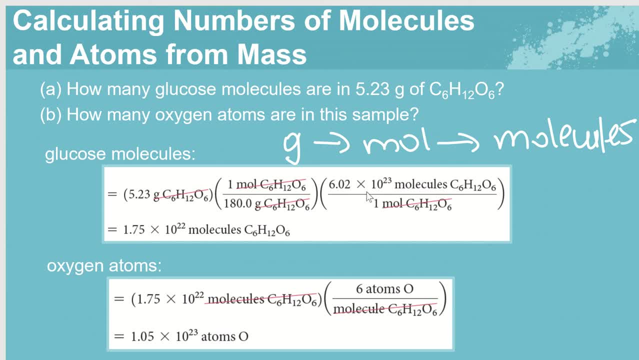 And so we have our two conversion factors here, Because we're going from grams to moles and then from moles to molecules. all right, So again, our given unit is grams and it's in the denominator. here, Our given unit is in the denominator of our. you know, this is our conversion factor. 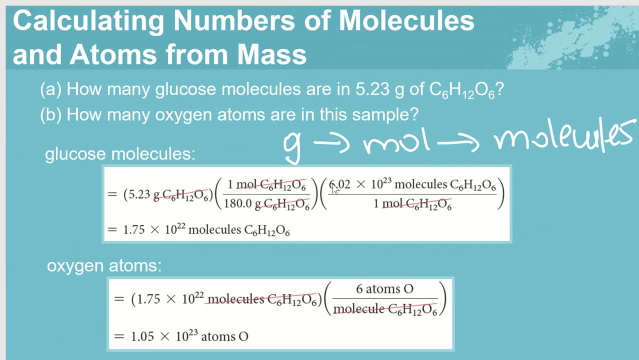 And for a second conversion factor. we're going from moles to molecules And so our given, Our calculated unit would have been moles from this step And we're trying to get rid of it. So it's in the denominator and what we 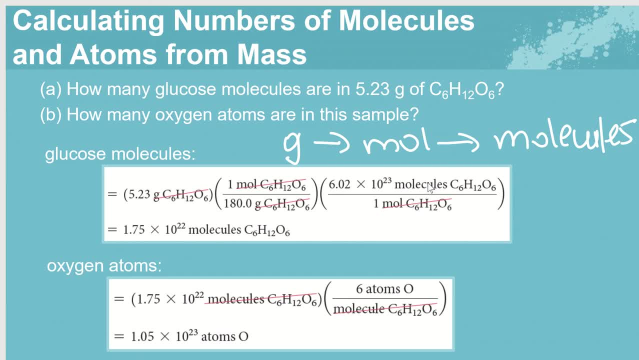 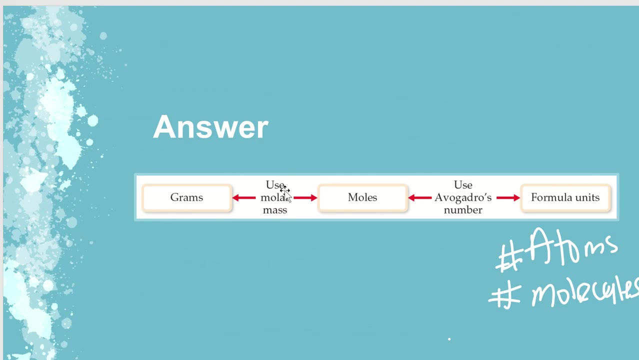 The unit that we desire is in the numerator right, So we'd go ahead and plug in these values. So this is our molar mass, remember? Let's go back to this. We need. We need molar mass to interconvert between moles. 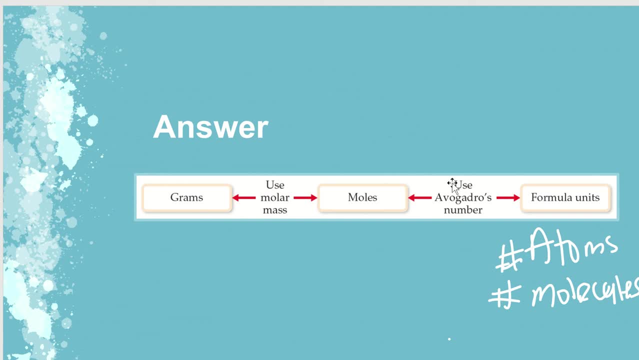 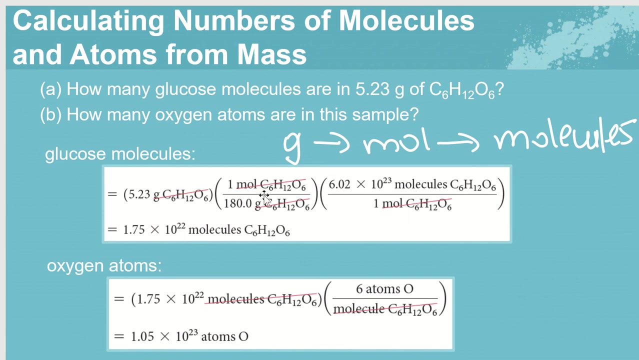 We need molar mass to interconvert between moles. We need moles and grams, We need Avogadro's number to interconvert between moles and either atoms or molecules, right, And so we just go ahead and do this calculation, do our multiplications, do our divisions. 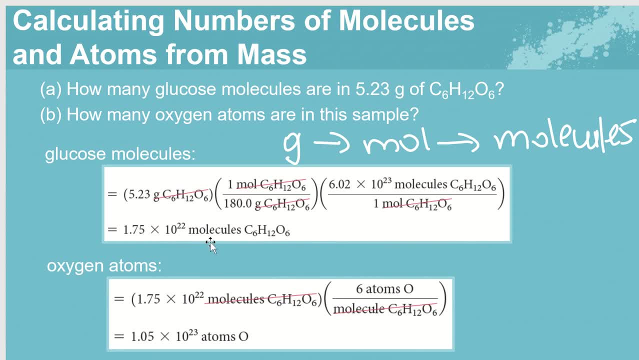 And then we should get 1.75 times 10 to the 22 molecules of glucose, right? So go ahead, Plug in these values And tell me if you get the answer For part B. it says how many oxygen atoms are in this sample right. 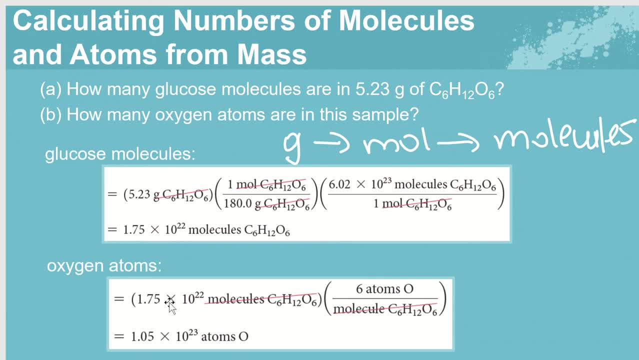 So here we're going from molecules to atoms, oxygen atoms in particular, right. And so we have a new conversion factor which says: one molecule Of glucose has six atoms, six oxygen atoms, right, And based on our molecular formula, here we're seeing that that is actually true. 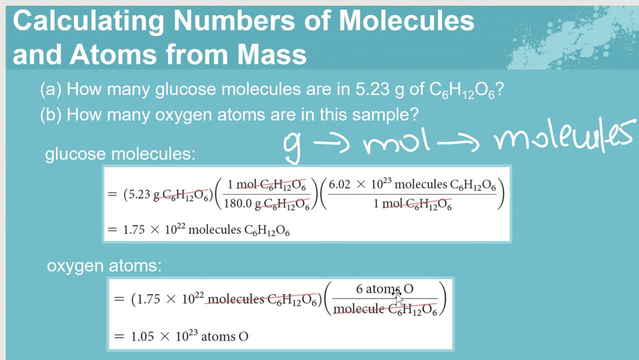 We have six oxygen atoms here, And so we have this very simple conversion factor And, you know, or the unit that we're trying to get rid of, you know, or given unit is in the denominator, So the desired unit, which is atoms, 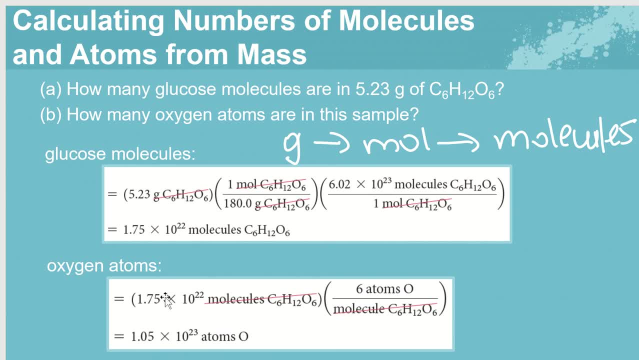 Atoms is in the numerator right, And so all we have to do is essentially multiply this number, or the molecules number of molecules, the number that we got from the previous question- by six in order to get the number of oxygen atoms right. 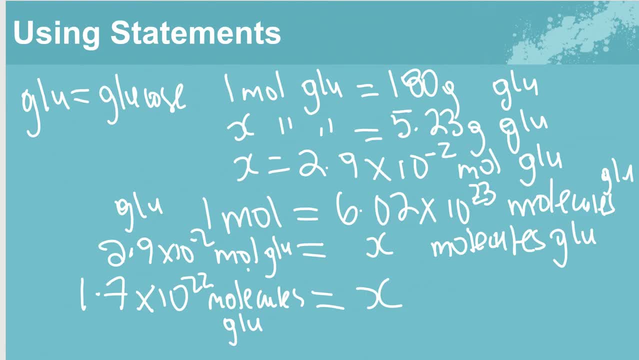 So, as usual, we like to use statements because that is the way we truly know if we understand what is going on here. So, as usual, we like to use statements because that is the way we truly know if we understand what is going on here. 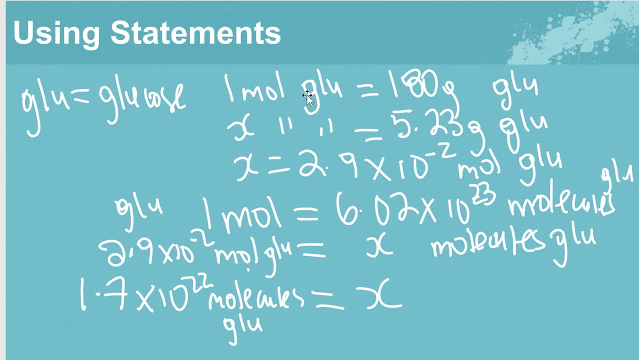 So in our first calculation we have our conversion factor, which is our molar mass right And, as I said before- I'm using a shorthand here- glucose, GLU right, All right, so just to repeat: right. 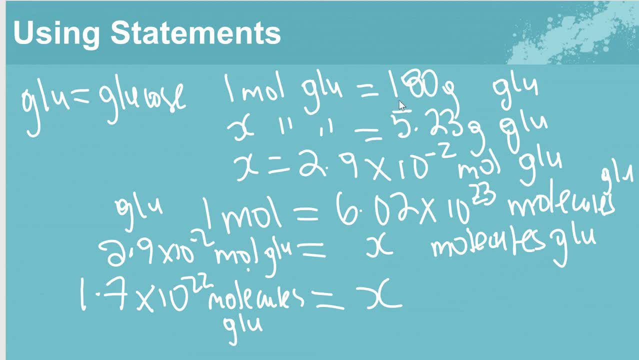 We have our conversion factor, which is our molar mass. remember, The molar mass is the interconvert between moles and grams, right. And so we cross, multiply and make x the subject of the formula, right. And once we do that, we get 1.7 times 122 molecules of glucose, right. 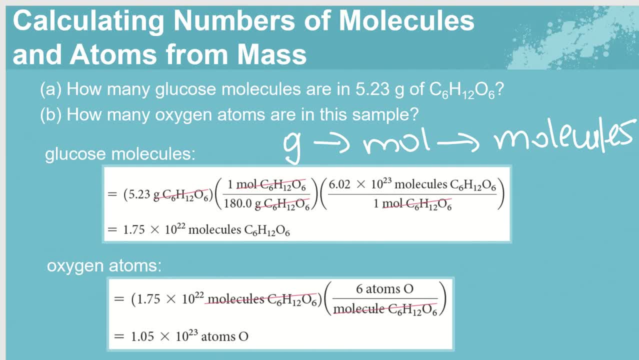 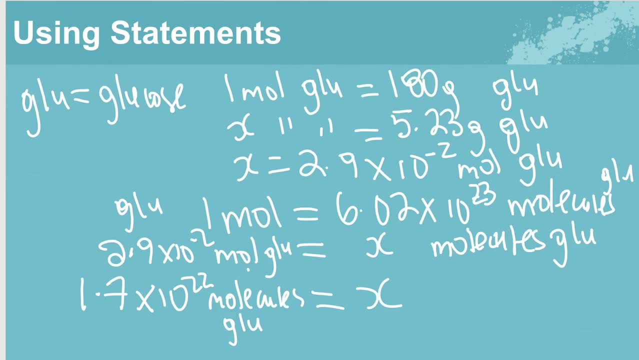 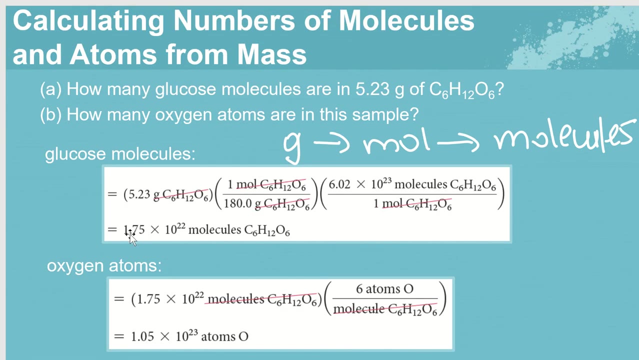 And that's the same number that we got here here, right. so notice here: you know we don't have the actual amount or the same amount of significant figures, so the correct number of significant figures would have been 1.75 or three significant figures. sorry, uh, based on the numbers that we have here, right. so when you are, 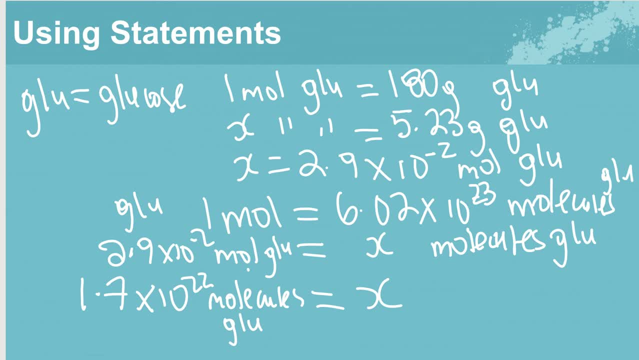 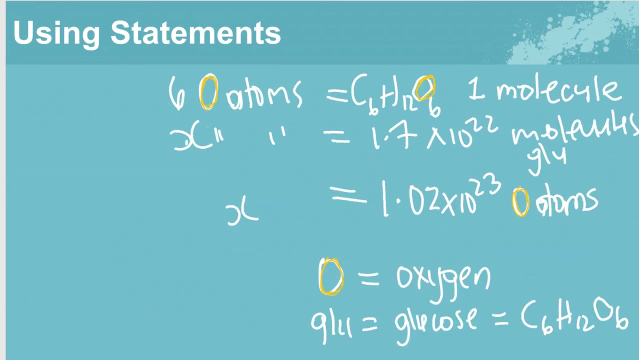 writing your um answer, ensure that you stick to the correct number of significant figures. right, but this slide is basically just to explain, using statements, the same calculation that we did before. right, and so for the second, for part b, in which we're asked to convert molecules to atoms. 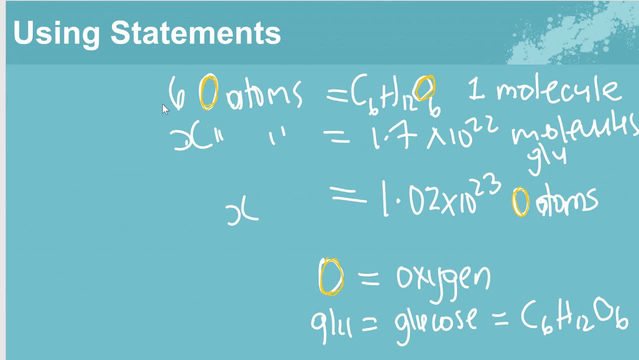 we have to write, or version factor, which is six oxygen atoms, is equal to one molecule of glucose. right, this is the molecular formula for glucose, and so here we have indeed calculated the number of molecules in the sample, which is 1.75 times 10 to 22 molecules of glucose. 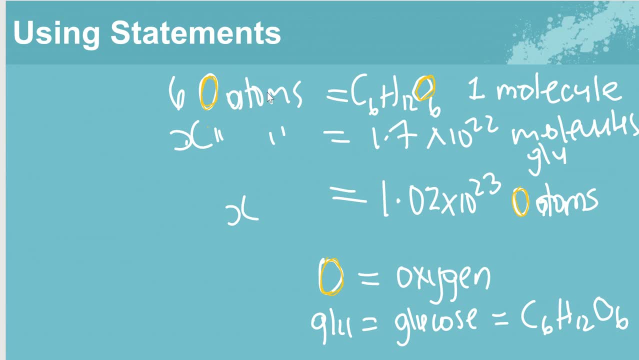 and essentially all we have to do here: cross, multiply or multiply by six, make x the subject of the formula, and then that works out to be 1.02 times into 23 oxygen atoms. right, so here you know these. just to have a little key here, this is: 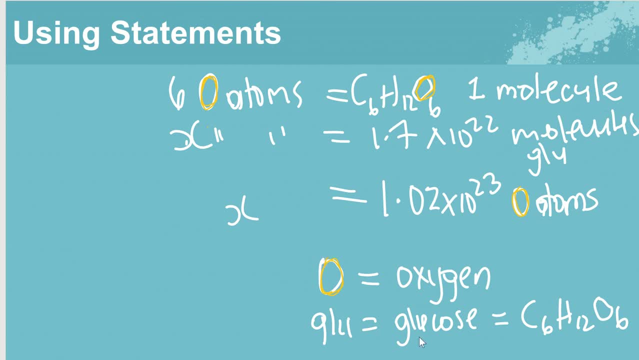 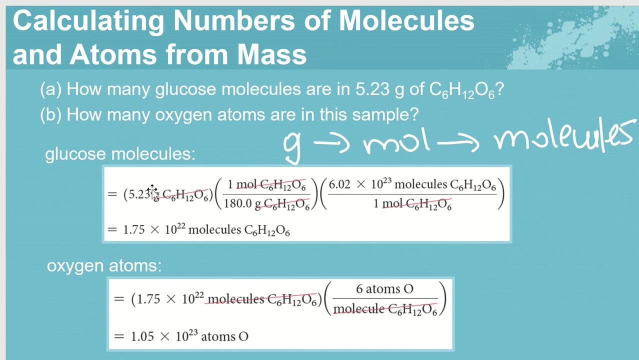 oxygen and, as we said before, glu, glucose and c6. that's equal to c6, h12, o6, right? so, essentially, guys, the point we're making, et cetera, right. so the key here is that we use molar mass to convert, to interconvert between: 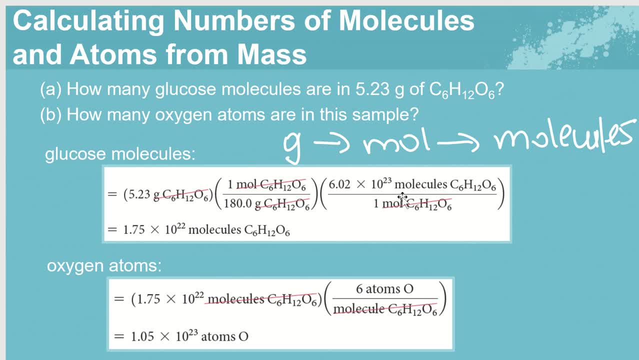 moles and its mass for itself. um, here we're going. this is so. this part is a little bit new. uh, so far we haven't really interconverted between uh molecules and atoms, right. so we just need to know here that one molecule of glucose, it has six oxygen atoms. that's our conversion factor, and once we multiply we get. 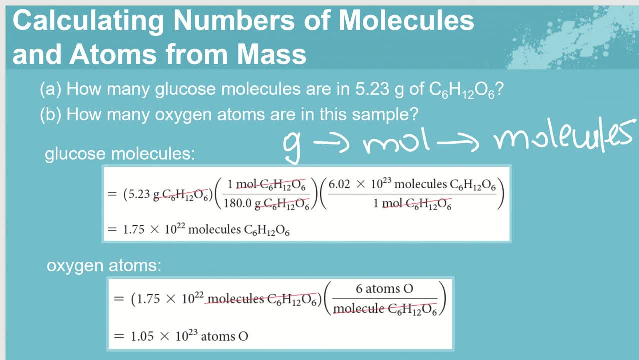 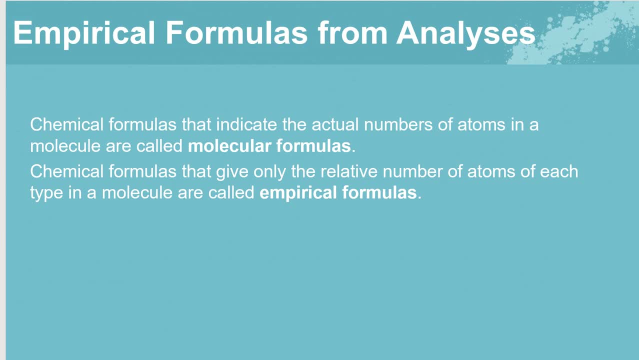 or number of oxygen atoms, all right. so the next thing that we're gonna talk about is or empirical formula- right, and how we use it, or how we get it from analyses. so chemical formulas that indicate the actual number of atoms in a molecule are called molecular formulas. 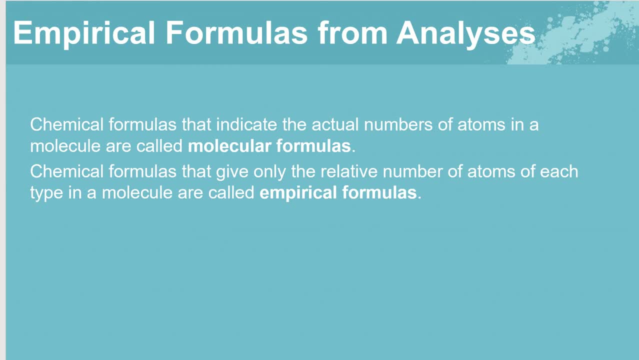 right. so, for example, or c6h12 o6 that we saw for glucose, that is, or molecular formula, chemical formulas that give only the relative- and perhaps i should have um underlined that word. it gives the relative number of atoms of each type of molecule. they are called empirical formulas. 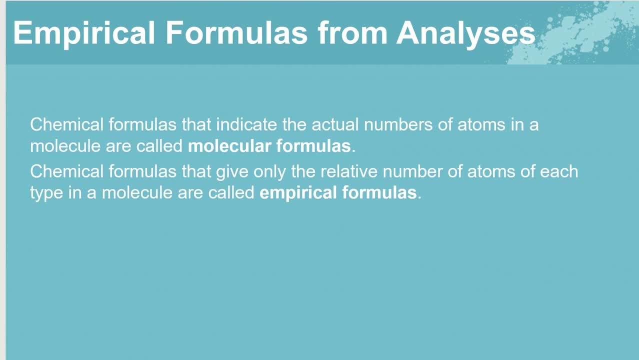 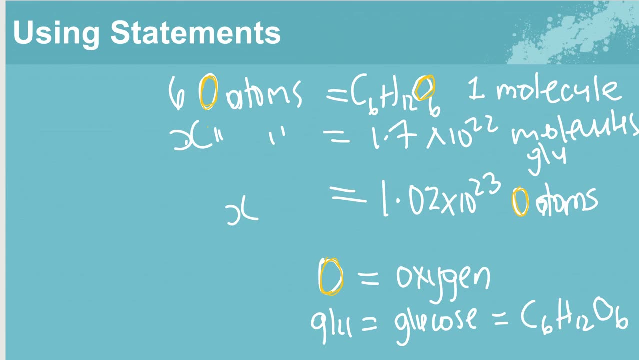 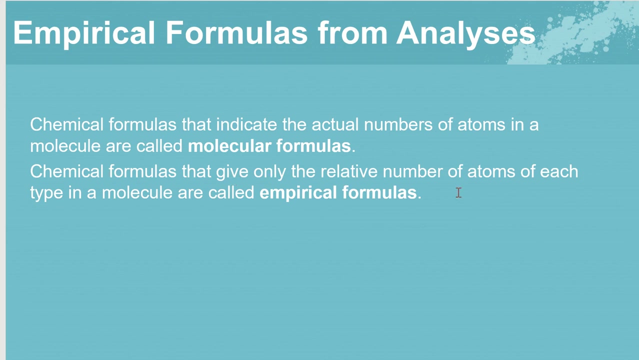 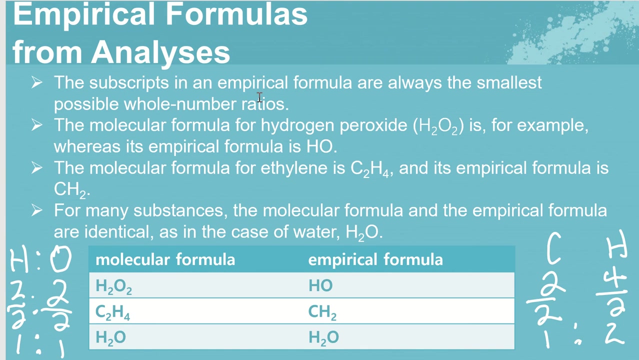 right, so what we just saw with glucose, c6h12, o6 here, that is our molecular formula and the form, chemical formulas that give the relative number of atoms. so we're going to see some examples of that coming up- are called empirical formulas. right, so the subscript in an empirical formula are always the smallest particles. 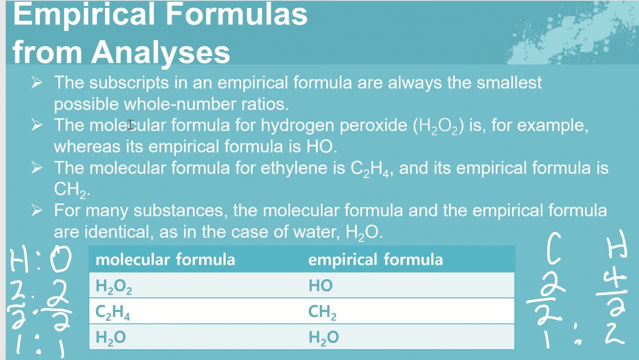 right, so we're going to see some examples of that coming up- are called empirical formulas. the molecular formula for hydrogen peroxide is h2o2 and, for example, whereas its empirical formula is ho, the molecular formula for ethylene is c2h4. its empirical formula is ch2. 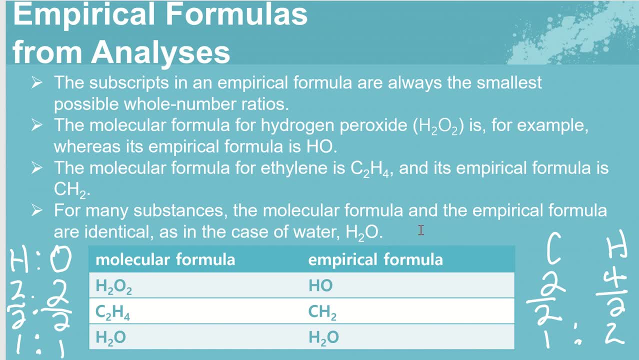 for some substances, the molecular formula is equal to the empirical formula, such as water, right, so we cannot go lower than h2o. so i have the same information in this table. here we have h2o2, the and the empirical formula ho, right. so what i want to highlight over here, let's 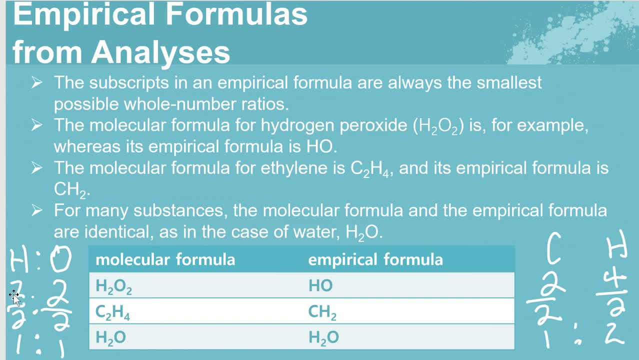 start with the um. we have two hydrogen and two oxygen and remember, when we're doing ratios, we want to divide by the lower or lowest of the two numbers. in this case it's lower and we- the two numbers here- are also the same, so we don't really have to use that rule. 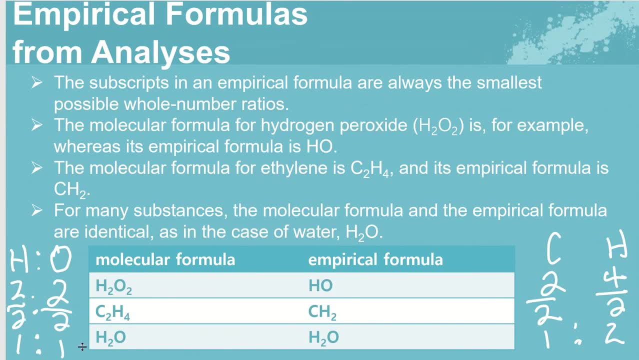 and so we divide through with the same number and we get a one-to-one ratio between hydrogen and oxygen, and that is why the empirical formula for hydrogen peroxide is ho. now for ethylene, we have two carbons and four hydrogens, and in this case the lower number is two. 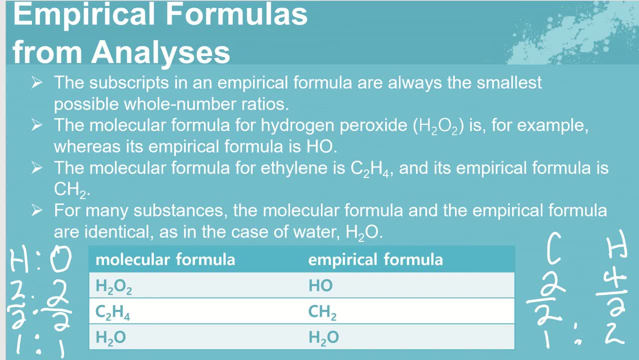 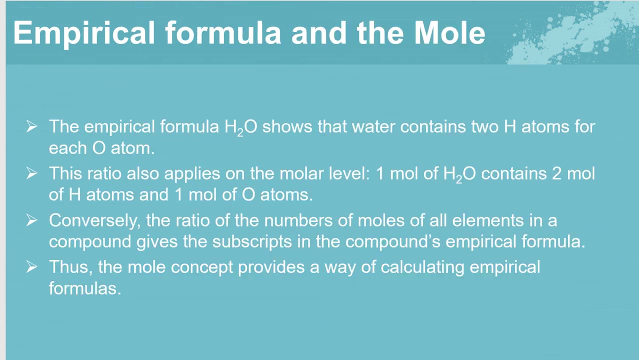 and so we divide through by two, and so we get a ratio of one carbon to two hydrogen, and so our empirical formula here is ch2. all right, so now we're gonna talk about empirical formula and the mole. so the empirical formula for water shows that water contains two hydrogen atoms. 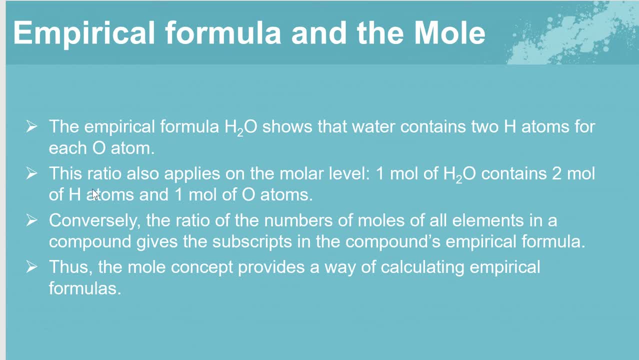 uh for each oxygen atom, and so this ratio also applies to on the molar level. so one mole uh- water contains two moles of hydrogen atoms and one mole of oxygen atoms. conversely, the ratio of the numbers of moles of all elements in a compound gives the subscripts. 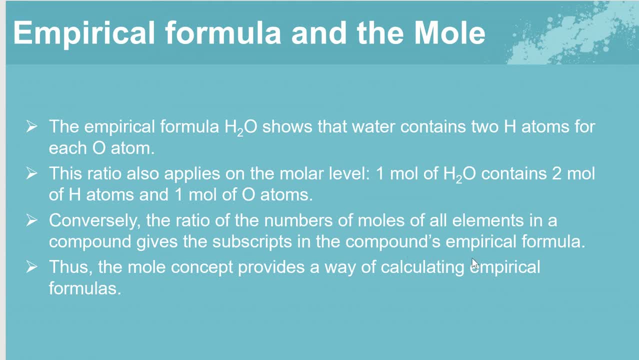 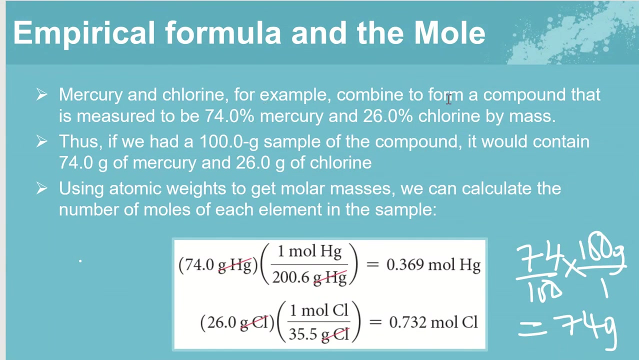 in the compounds empirical formula. thus the mole concept provides a way of calculating empirical formulas. let's try to make that a little bit clearer. so here we have mercury and chlorine, for example. they combine to form a compound that is measured to be 74 percent mercury and 26 percent chlorine by mass. 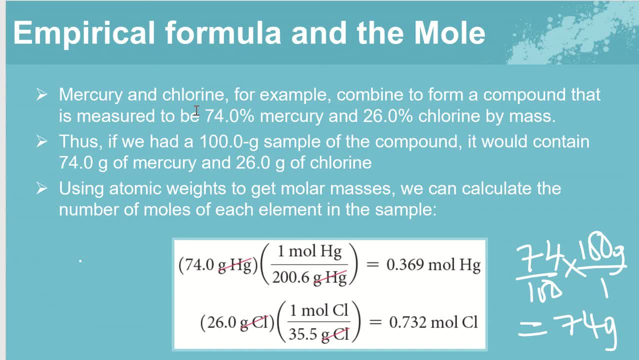 right and so if- and underline the- if- we had 100 grams, a 100 gram sample of the compound, it would indeed contain 74 grams of mercury and 26 grams of chlorine, because if we have 74 percent, that means 74 divided by a hundred times a. 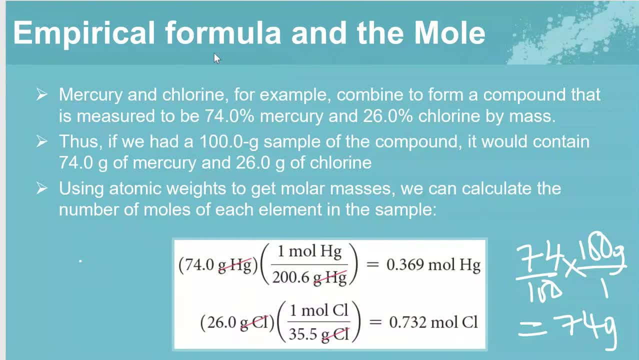 hundred equals the same thing, right? so if we had a different sample, if it wasn't 100, a 100 gram sample, then we would have to do this calculation in order to calculate the number of grams. but we're keeping it simple and so, using this formula, we're going to calculate the number of grams we're going to use. 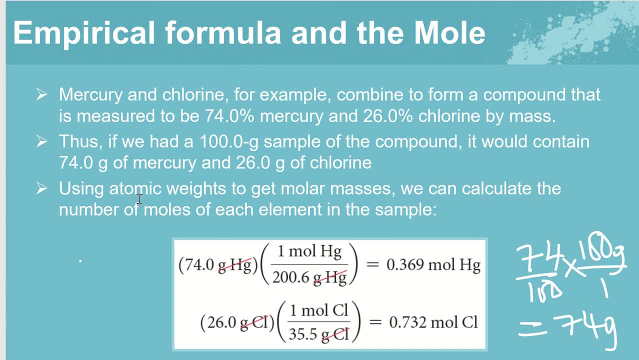 this formula. we're going to calculate the number of grams. we're going to use the atomic weights to get molar masses. we can calculate the number of moles of each element in the sample right. so again, what did we say? what number do we use to convert grams to moles? well, if you had molar mass, then you are indeed. 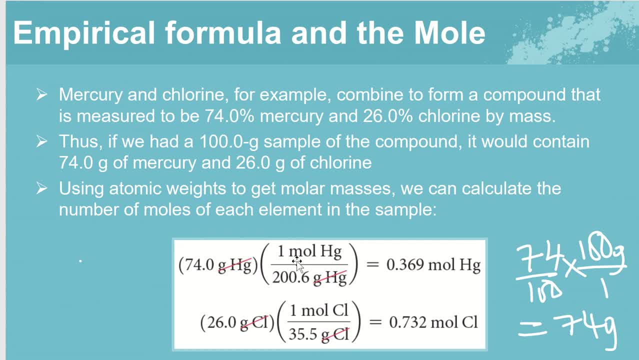 correct. or if you said molar mass, that's correct. so we need to look in our periodic table to calculate the number of moles of each element in the sample, to find out the atomic weight for mercury as well as for chlorine, right. so that's where we would find these numbers right and all numbers you know related to. 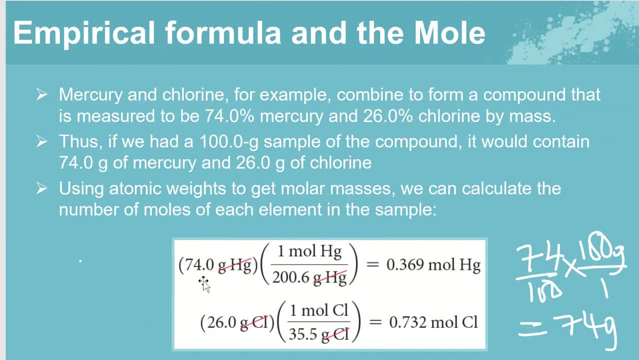 the molar mass right, and so here, or given unit is 74 grams, and so that is in, or denominator of our conversion factor, and we divide and we get the number of moles. here for the second part of the calculation, for the chlorine, we're converting grams to moles again, and so we divide it through and we get to the 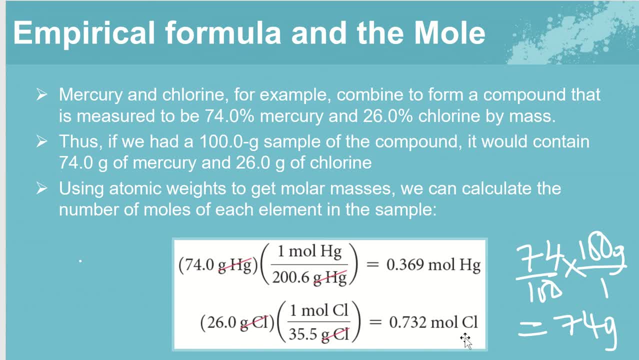 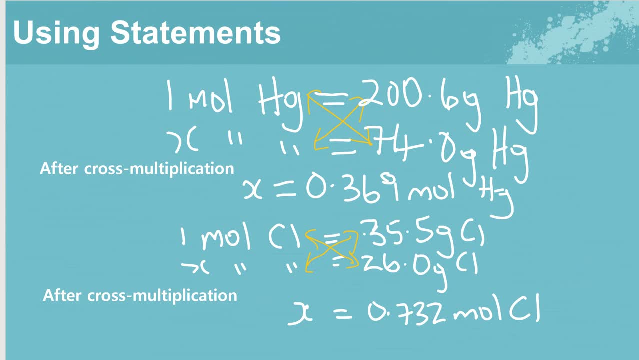 number of moles of chlorine. right, okay, you, and so, as usual, we like to look at the statements. right, and so we have: one mole of mercury is equal to 200.6 grams of mercury, and so we're trying to find the moles. you know, cross, multiply, make X the subject of the formula and we get the. 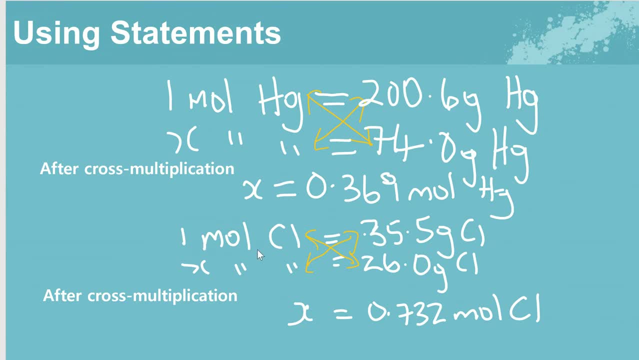 number of moles and the same for chlorine. one mole, chlorine, is equal to 35.5 grams, and so we're trying to find how much is in 26 grams. okay, so if you're interested to get the chef's Magazine, check out our chacun. 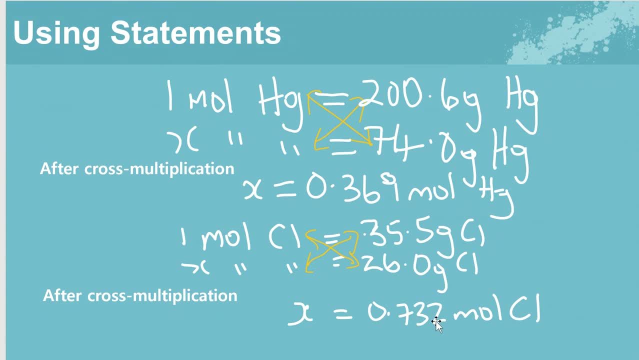 YouTube channel bar or exit page and again you- and if you have any questions on our section over here, you have that question here- you can drop us a line under those video sharing for help us in this question. so please do during the conversation we're going to take very briefly and then start from the 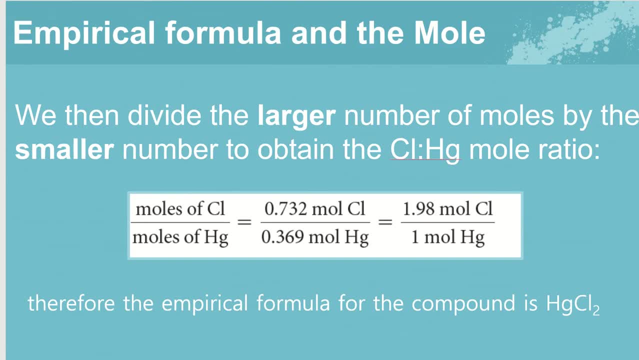 second part of this lecture, you know, and then maybe just give you some ideas on how exactly this curriculum. so obviously, if you're watching now this particular lecture, you also get to do the calculation and theazed with us. so here we go. ratio, right, so. so here we divide the moles of the, the lower number, right? so where the two numbers. 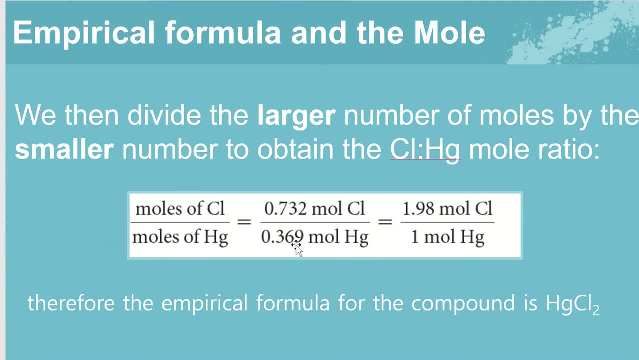 that we're looking at is 0.369. uh moles of mercury right, and then we. the second number is 0.732, so the lower number is the 0.369 and if we divide through by the smaller number we get a ratio of: 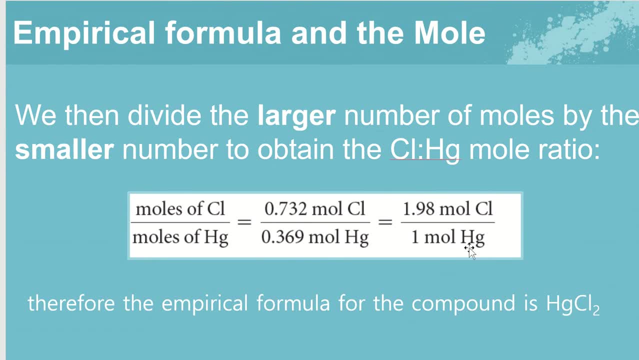 one to two. so just go ahead and plug in these values and work along with me and let me know if you get the same answer one to two. and so if we got the same answer or empirical formula here of compound, of the compound in the question, you can see that the ratio of one to two is 0.369. and if we divide through by the smaller number, 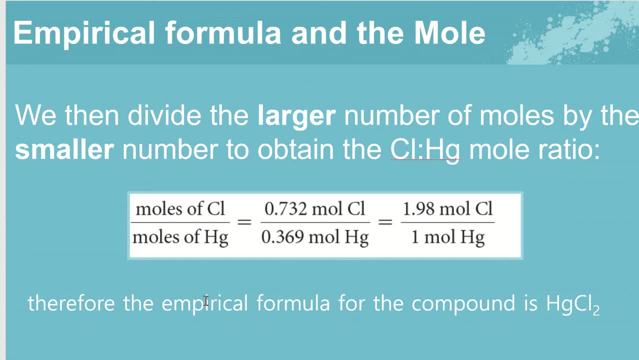 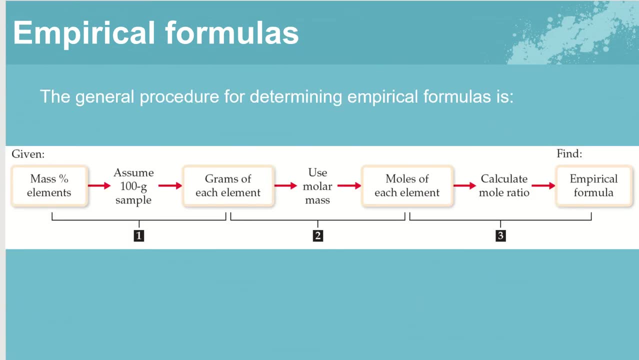 is hgcl2 because of the ratio that we calculated here, and so the general procedure for determining empirical formula is this right. so we're given the mass percentage of the elements right, and we assume that we have a 100 gram sample, and so we basically just change a percent to grams because of this assumption. and that is step one. step two says: 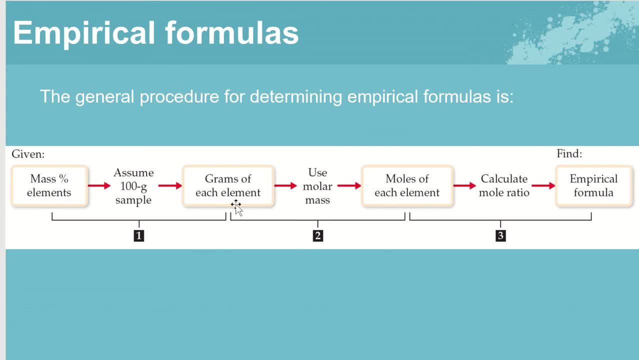 we convert the grams to moles, as we say and as we saw, sorry, and then to do that we need the molar mass, and that is step two. once we calculated, or once we have the moles, that leads us to step three, which means we calculate the mass of 1.3 to 1.3, and that is step one. once we calculate 2.3, that leads. 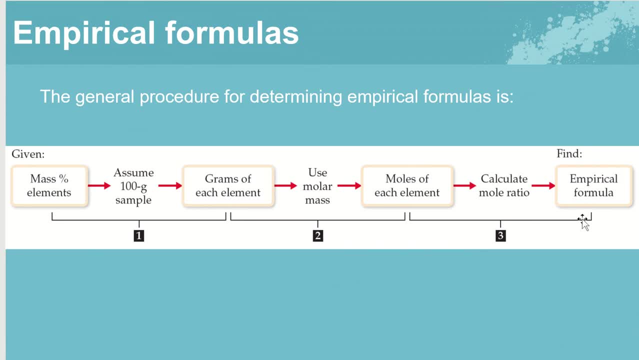 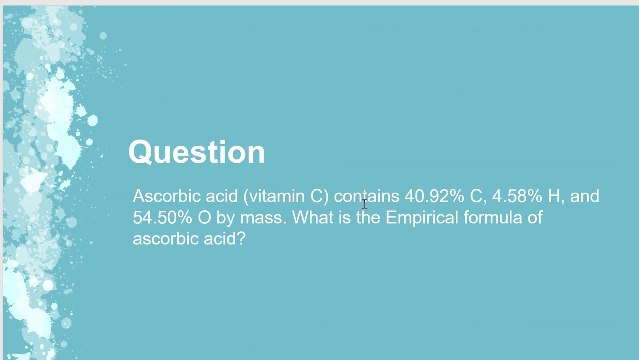 means we calculate the mole ratio and so we get our empirical formula. so let's see if you were following our question here. says ascorbic acid, which is vitamin c. it contains 40.92 percent carbon, 4.58 percent hydrogen and 54.50 percent oxygen by mass. what is the empirical formula? 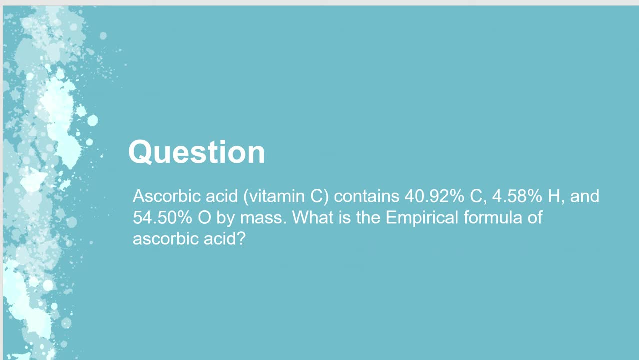 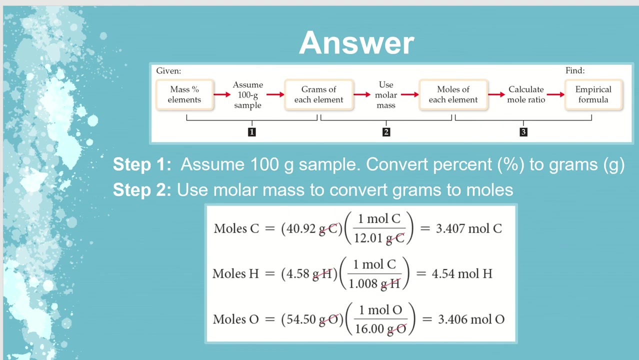 of ascorbic acid. all right, so i would love if you take a second to try to attempt the answer before you look at it. all right, so that's how we learn. all right. so here you know. just a reminder of the general procedure. so step one says: assume that we have a 100 gram sample. in that way we convert our percentages. 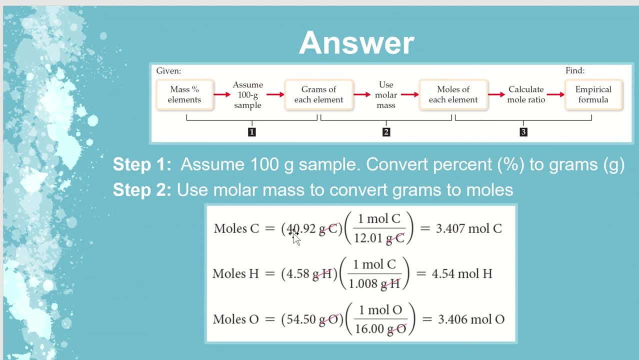 to grams, right? so we're given 40.92 percent, 4.58 percent and 54.50 percent. so if we assume that we have a 100 gram sample, we're given 40.92 percent and 54.50 percent. so if we assume that we have a 100 gram sample, all we have to do is to just change our percent. 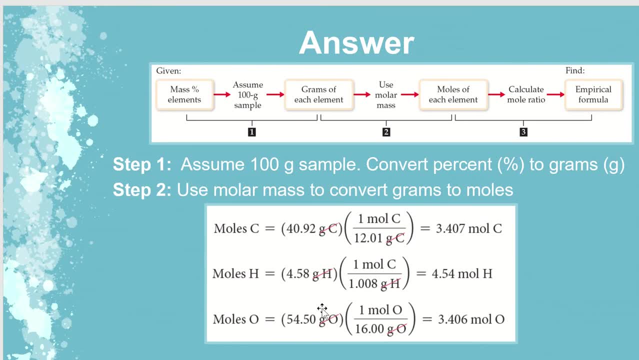 to grams. that's the first step, or a second step is to use the molar mass to convert grams to moles. right and so here, this is what we have, here we're convert, we have our molar mass of the different elements and we converted our grams to moles. 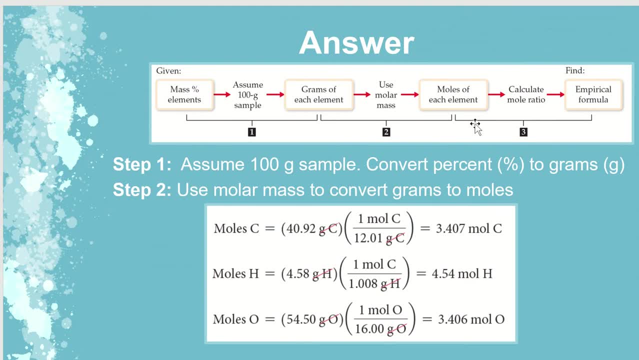 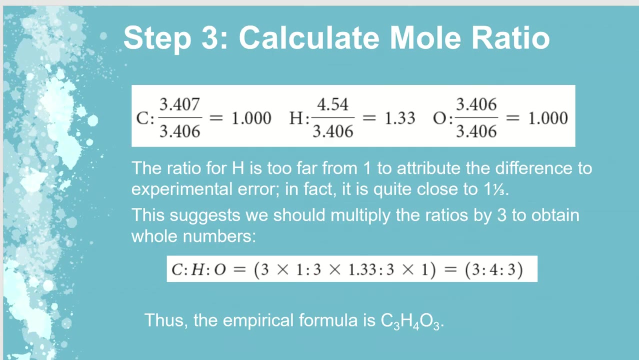 as we have seen previously. so what's the third step? the third step is to calculate the mole ratio, and therefore we get the empirical formula all right. so since the smallest value is 3.406, we divide through by or small less number, right, and so we get a ratio of one to one point three. three to one, right, and so. 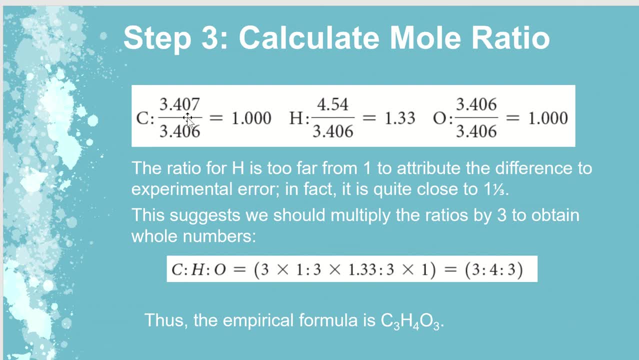 notice our significant figures right. so here we have four significant figure. the answer is four significant figure. the here we have the lowest significant figure is three. we have three significant figures here. so the ratio for hydrogen is too far from one to attribute to the difference in experimental error. so the what happened is that recall when we had? what was it here, right? 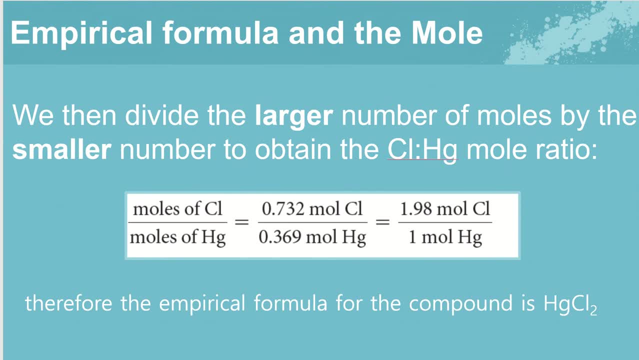 here we had one to one point, nine, eight, and we basically rounded up to two, right? so we're saying, let's say we traveled a range of two different values to each of the corresponding ratios and then the ratio in between that. huh, there may be, may have been, some experimental error, and so 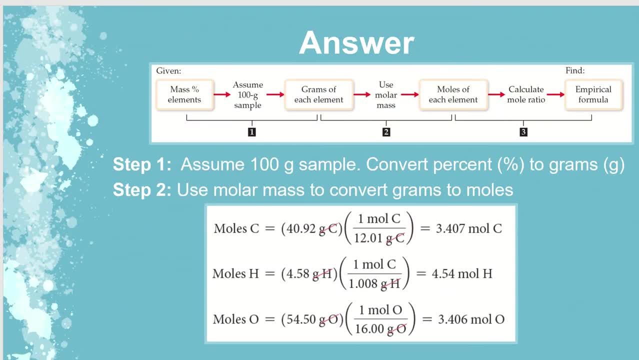 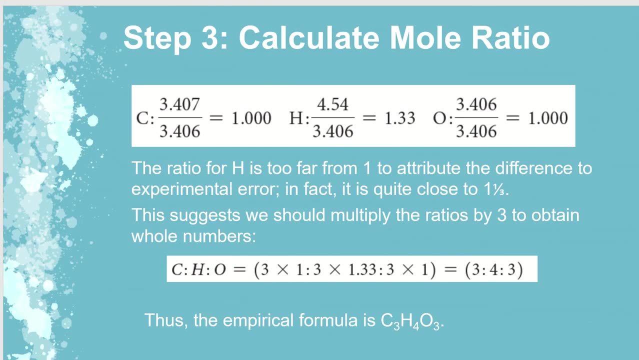 we're going to round up to two, one point nine. eight to two. however, in this case, we're saying that 1.33 is too far from one Round up. we cannot basically say that it's one right. In fact it's quite close to one and a third. 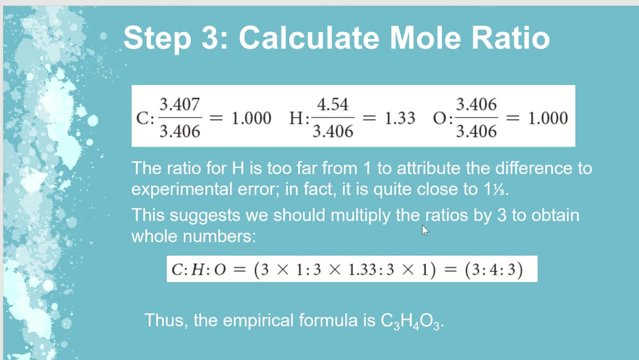 And so because of that, it is suggested that we multiply the ratios by three to obtain whole numbers, right? So three times one, three times one and a third and three times one here, Right? And if we do that we'll get a ratio of three to four to three, right? 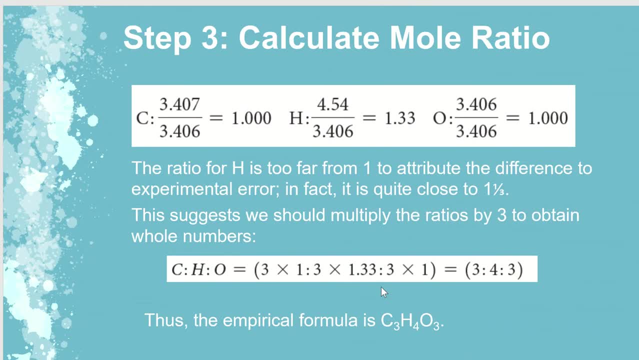 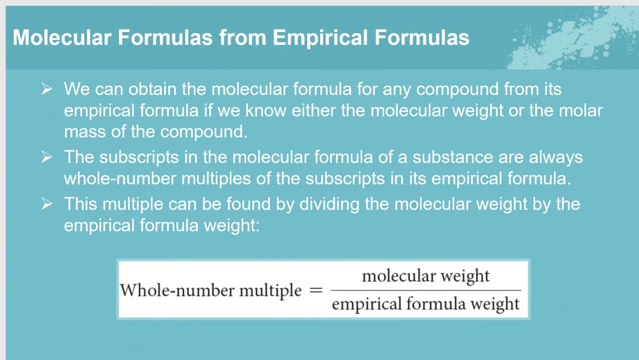 And that is our empirical formula. All right, so what's the point in getting an empirical formula if we cannot convert it to our molecular, Molecular formula? So how do we do this? Well, we can obtain the molecular formula for any compound from its empirical formula if we know either the molecular weight or the molar mass of the compound, which is basically the same thing, right? 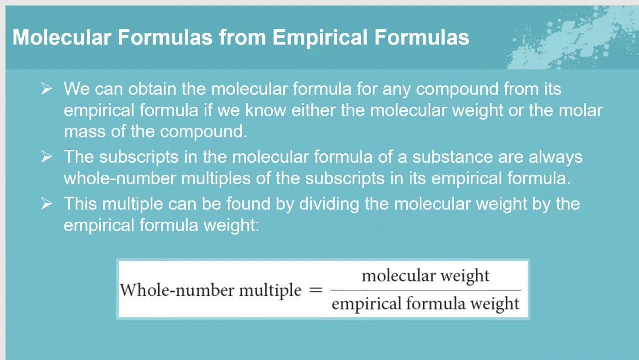 And so the subscripts in the molecular formula of a substance are always whole number multiples of the subscript. So what we want to do here is to find the well, we're given normally the molecular weight, and we know what the empirical formula is, so we can calculate the formula weight of the empirical formula, right? 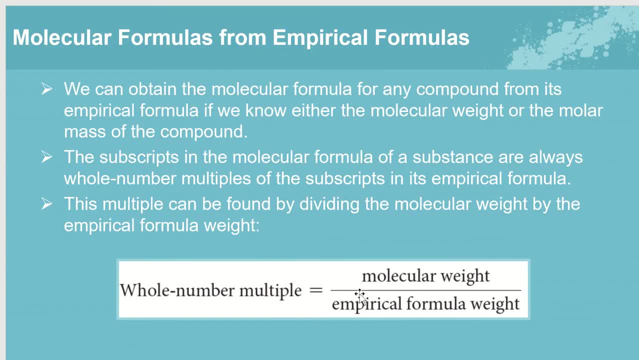 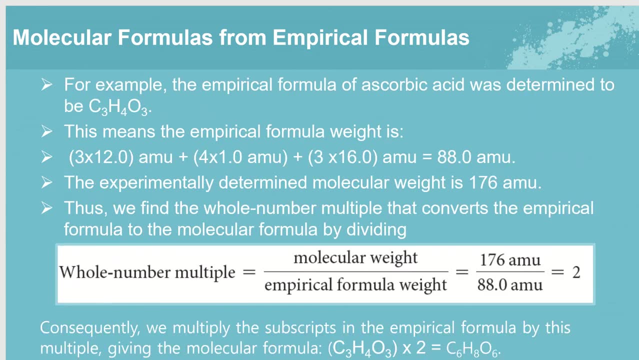 And then divide that by the molecular weight And then divide them as we see in this equation here to get the whole number multiple. Let's see if we can make it a little bit clearer on this slide. So, for example, the empirical formula for ascorbic acid was determined to be C3H4O3, right? 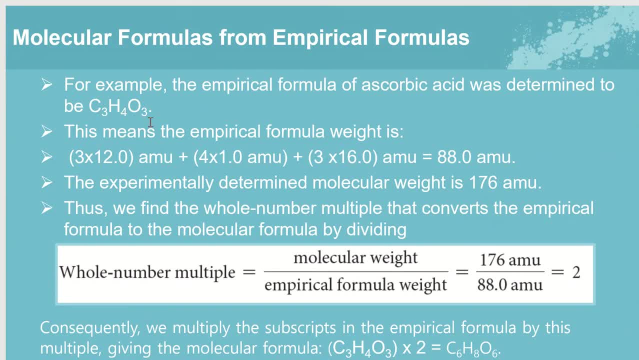 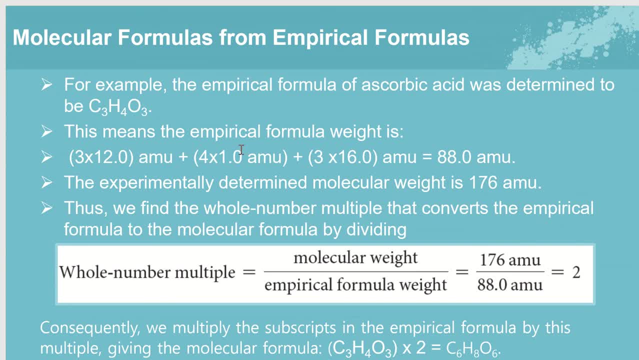 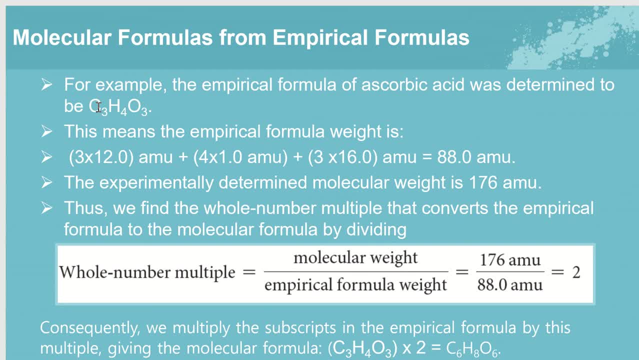 know carbon, hydrogen and oxygen, the atomic weight, Or we can say atomic mass units, Right? It's 12 for carbon, and so three times 12 plus four times one for hydrogen, plus three times 16.. 16 for oxygen and we end up with the empirical formula weight to be 88 atomic mass units, right? 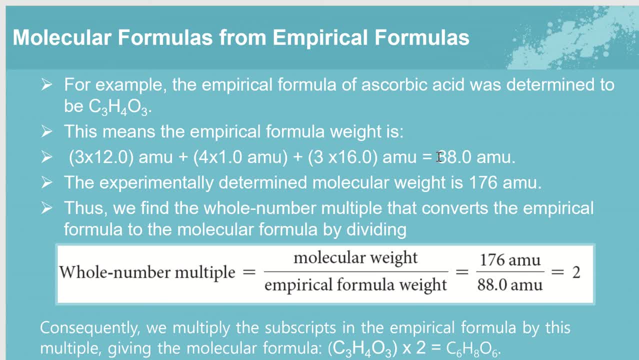 and so the experimentally determined molecular weight is 176 atomic mass units. and so we're given the molecular weight. and so to find this whole whole number multiple that we speak of, we just divide the numbers by each other, as we as we see here, which is 176 divided by 88, and we get 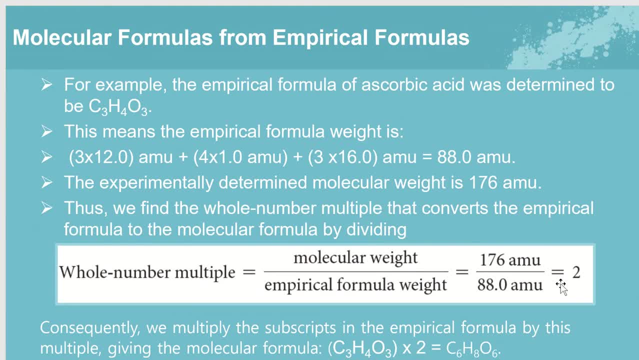 2. consequently, we multiply the subscripts in the empirical formula by this multiple in order to get the molecular formula right. so 2 times 3 gives us 166, two times four gives us eight, and two times three again gives us six. so we have therefore: 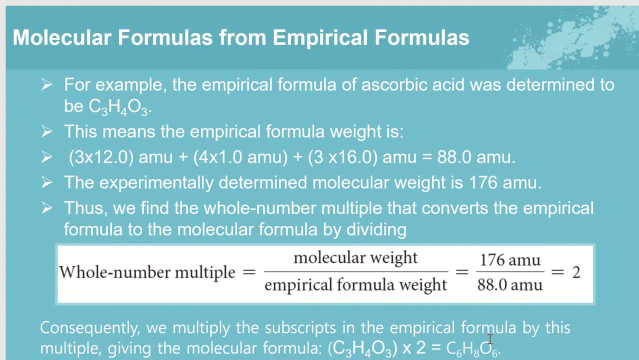 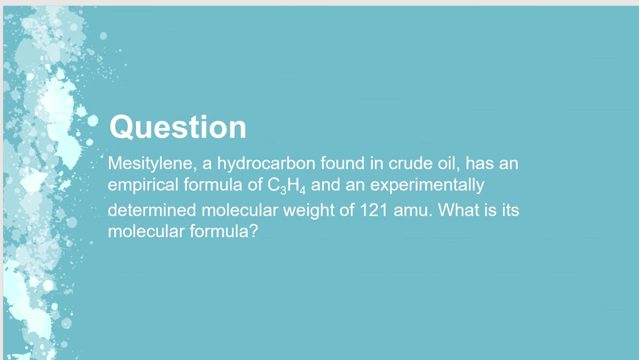 successfully converted or empirical formula to or molecular formula. alright, so let's see if we understand what's going on. mesethylene, a hydrocarbon found in crude oil, has an empirical formula of c3h4 and, and, and then experimentally determine molecular weight of 121 atomic mass. 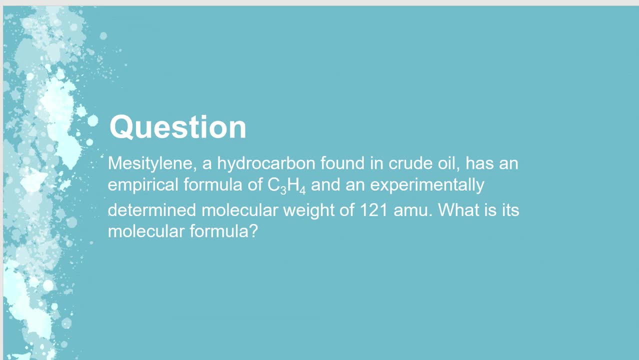 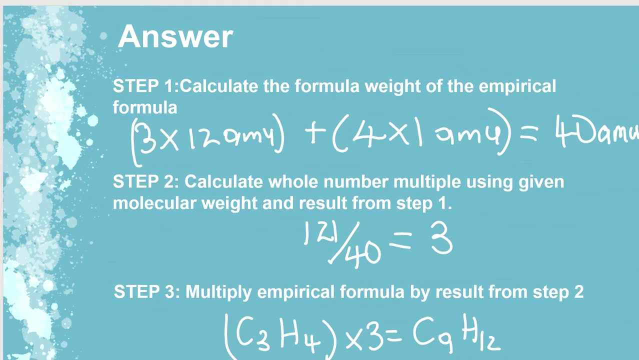 units. what is its molecular formula? so this is how you know, if you understand, if you can go ahead and do the calculation before looking at the answer. all right, so we have three steps, right? so the step one is to calculate the formula, weight of the empirical formula. so it's c3h4, and so 3 times 12 plus 4 times 1 gives us 40. 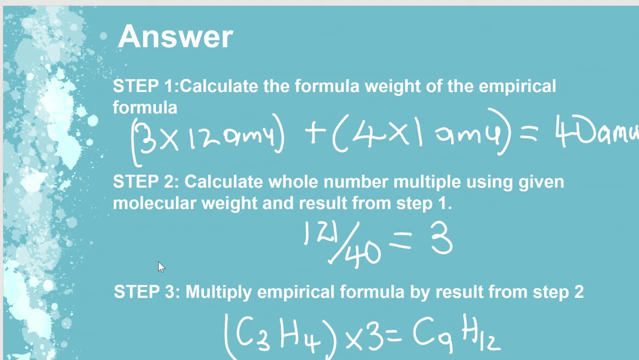 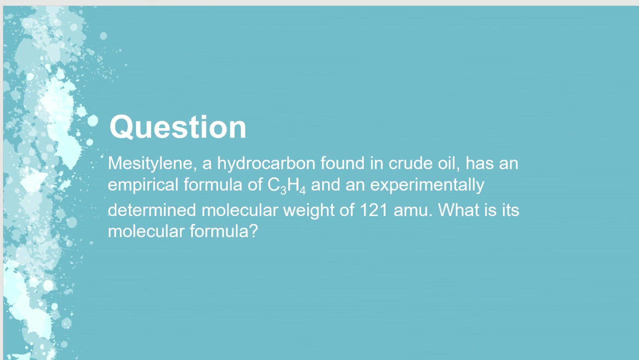 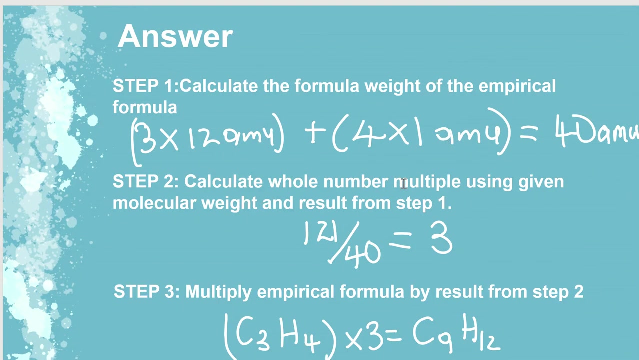 atomic mass units. and then step two is to calculate the whole number multiple using given molecular weight and result from step one. right, and so our given molecular weight in the question was 121 atomic mass units. and so we divide that by the answer from step one and we get the- uh, the number or the result to be 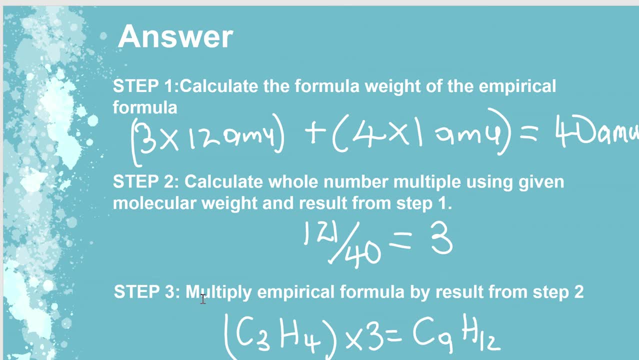 three, and then our final step is to calculate the whole number multiple using given molecular weight, is to multiply the empirical formula by the result from step two, which is three. right, and so we're given the empirical formula, which is c3h4, and therefore, if we multiply by three, so three, three is